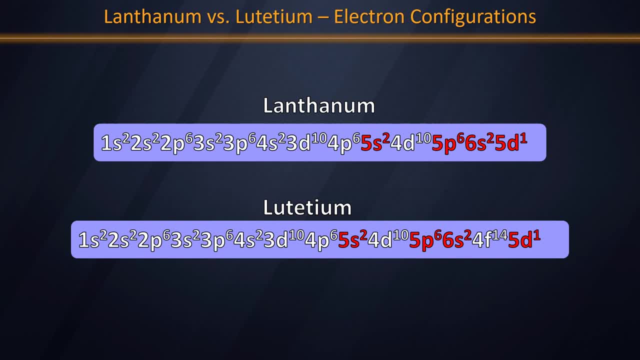 but also even the same interior configuration. as far as their fifth principal energy level is concerned, There are 5s2, 5p6, 5d1.. So is lutetium: 5s2, 5p6, 5d1.. In fact, 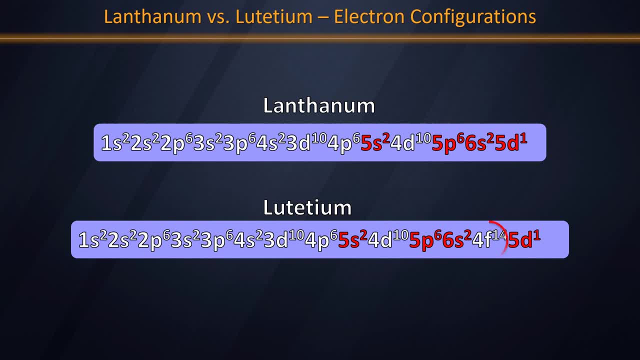 they only differ substantially by the filling of that 4f subshell, and indeed the entire series between lanthanum and lutetium represents elements in which the 4f subshell, by and large, is the one that's being populated by the additional electrons necessary. 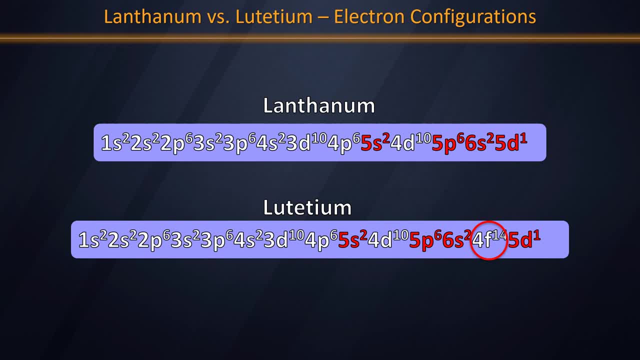 to compensate for the increased nuclear charge of the nucleus in each of these elements. So why is it that adding 4f electrons doesn't really do much to the chemical and physical properties of these elements? Well, let's consider that once again in the context of lanthanum. 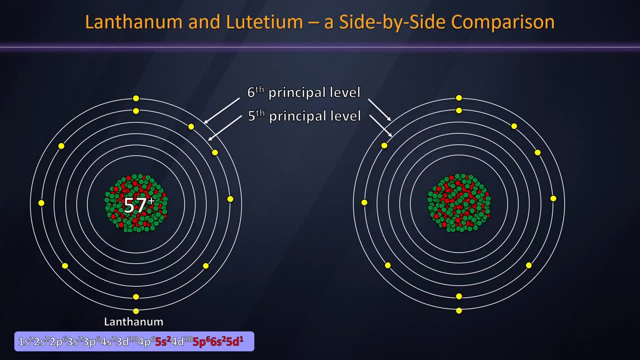 and lutetium. Okay, so here is a Bohr model of lanthanum. Now please forgive me for using a Bohr model for such a complex chemical argument here, but I promise you it's actually going to get the job done here. I know it's very simplistic, but this is a Bohr model of lanthanum on both sides. 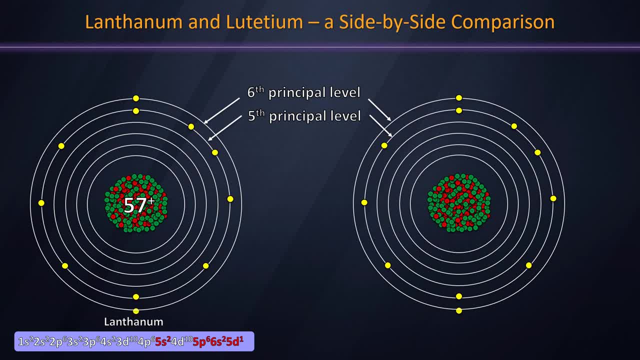 of the screen at the moment, with its 5s2,, 5p6,, 6s2, 5d1 electron configuration in its outermost two energy levels, and we're going to represent all the remaining electrons that are in the 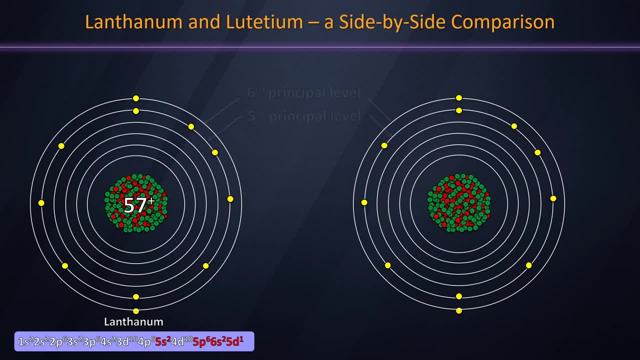 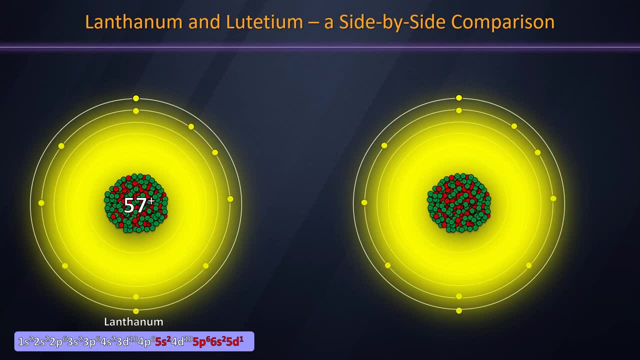 remainder of these interior levels here as just kind of a yellow mass, because they're so deep within the atom. they really don't have anything to do with the face that the atom presents to the world and therefore how those atoms interact with the world. Now, in order to change lanthanum, 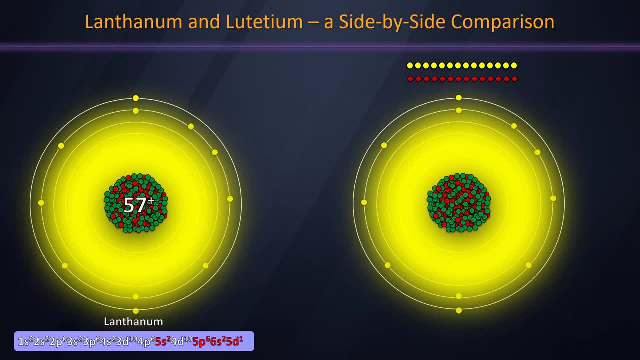 to lutetium, we're going to have to add 14 protons and 14 electrons and of course you will have to add additional neutrons, but we're going to leave those out because they're not really germane to that we're going to make today. Remember, lutetium has those 14 additional electrons. 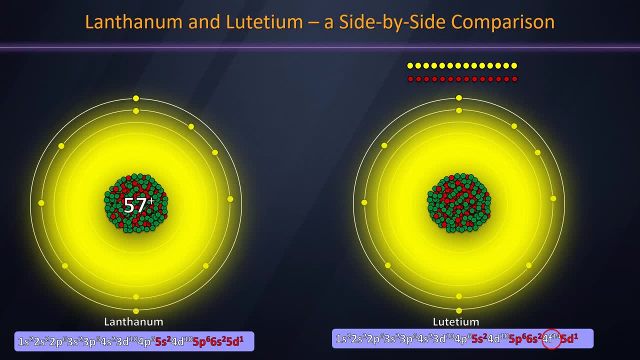 stored in the 4f subshell. There are two important things to remember about the 4f subshell. First is that it's in the fourth principal energy level and that's deep within the electron cloud of that atom, and second is that f subshell electrons are absolutely terrible at screening.